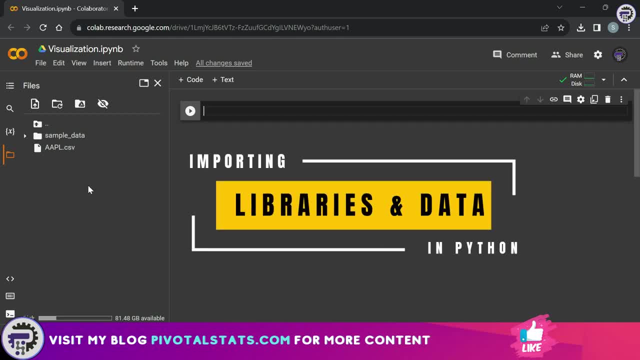 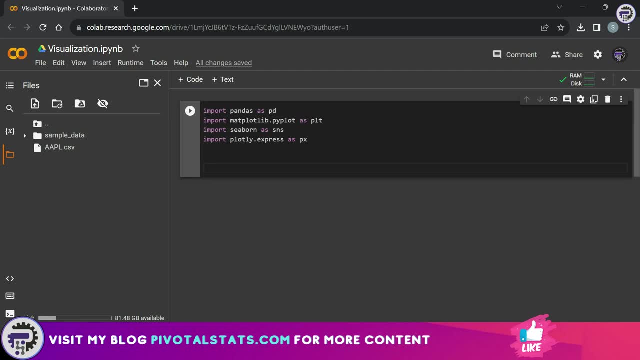 Now, since I'm using Google Colab, I'm going to directly import it, because it's already been installed. Now, after importing all these libraries, I'm going to just copy paste the path from here, Okay, And also create my data frame. 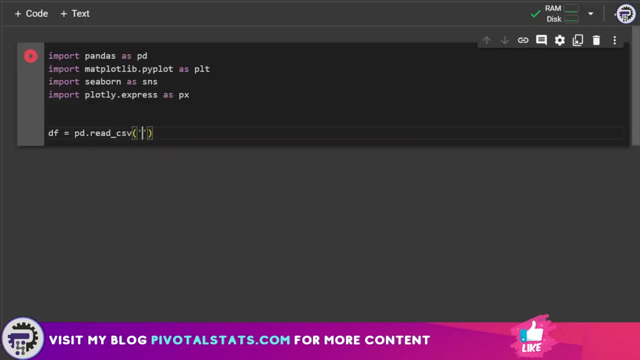 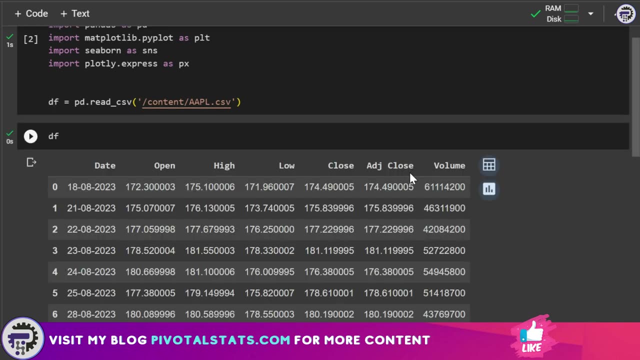 Now let me just quickly show you the dataset. So in this data we have a date column open, highest point of our stock for a day, lowest closing price, adjusted closing price and then volume. Before we move forward, I'm going to convert this date column to a date time format. 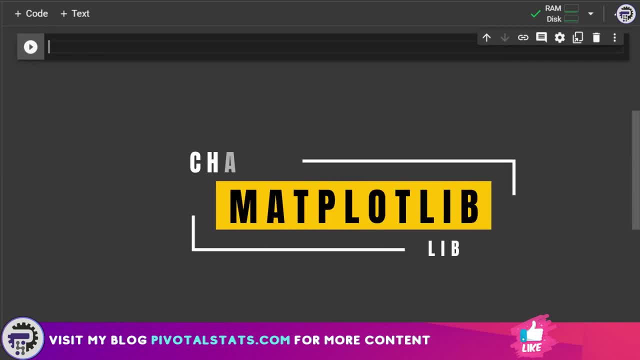 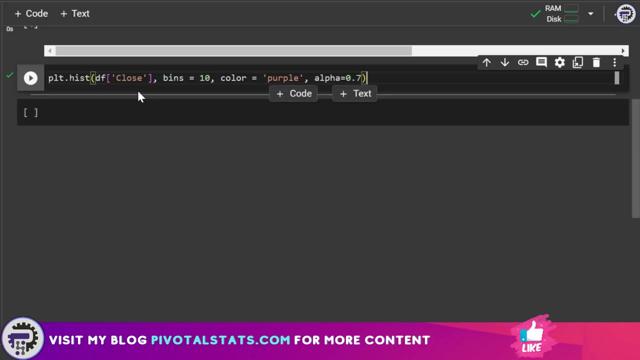 Okay, Once that is done, let's start creating our matplotlib charts. To start with, let's start creating a histogram. Okay, So I'm going to say plthist. Now let me just quickly explain the parameters that I've used in plthist. The first one is the column that I'm going to use to create that histogram. 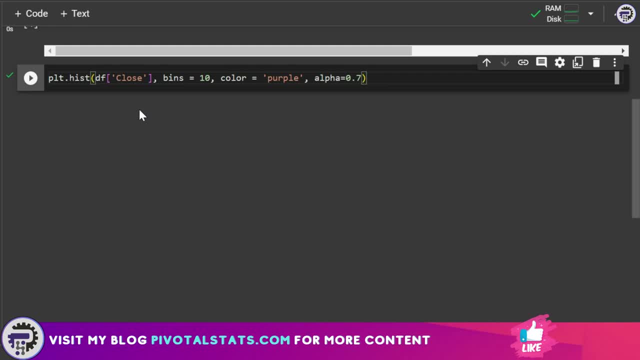 So for this I've used the closing price column Bins is nothing but the width of the data points that I'm going to present in that particular histogram. I'm defining a standard color for my chart, which is purple, and then the alpha value, which represents the transparency of a certain 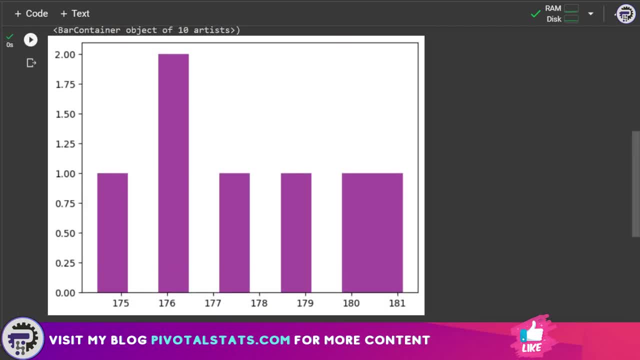 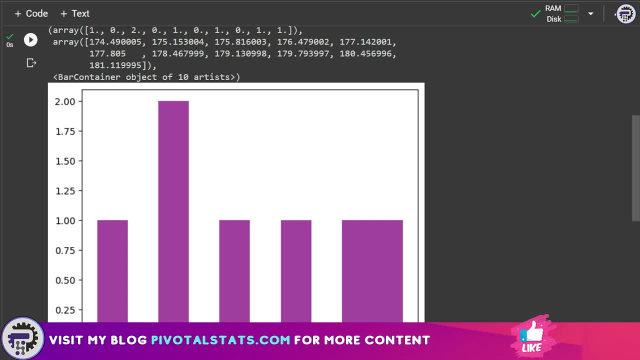 chart. So if I run this as it is, it's going to give me a normal chart like this. However, as you see, I do not have any labels in this chart or titles in this chart. In order to add labels and titles, we have to use certain additional methods. The first one is to add a 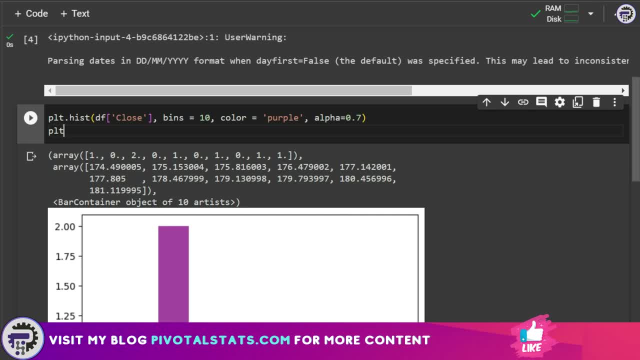 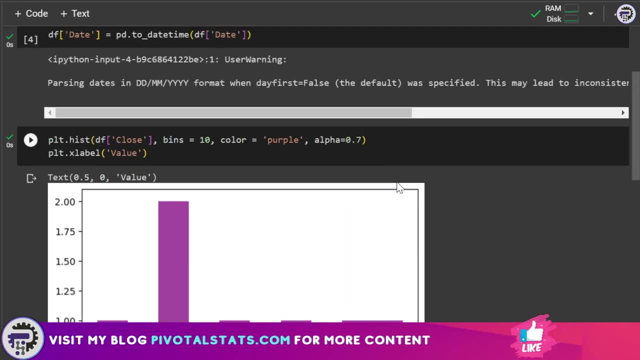 label in my x-axis, So I'm going to use pltxlabel. Now, if you see, it has mentioned value here and you can use any text that you want. Next one is to add a label in the y-axis, So I'm going. 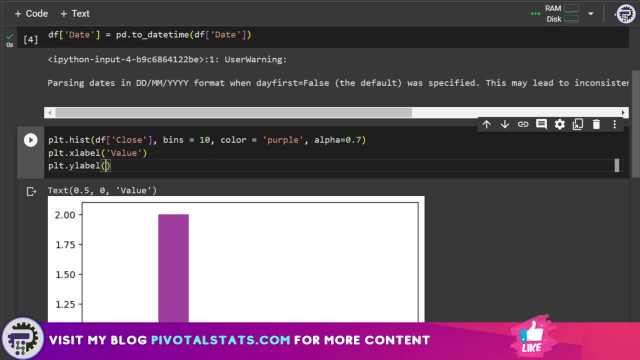 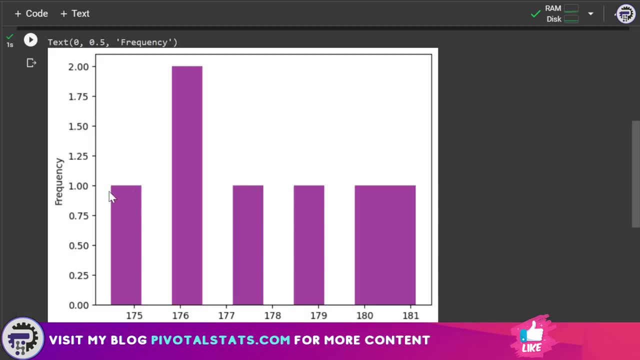 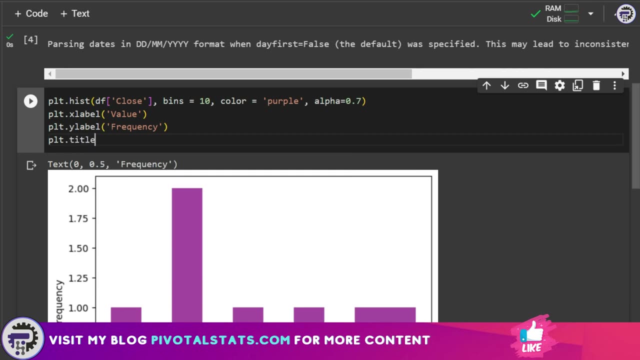 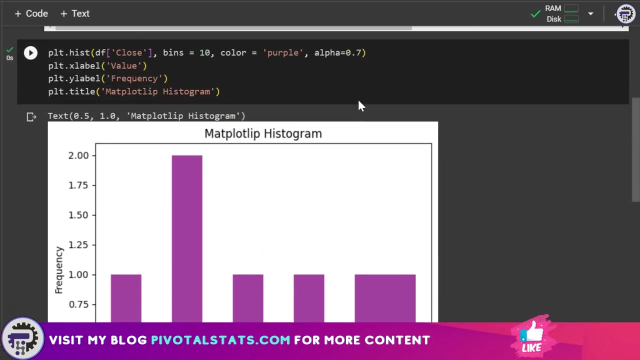 to use pltylabel. Let's say frequency, So it has added that label here. Then let's add a title to my chart, So plttitle, So it has added a title here. Now, as a best practice while you're displaying a chart, 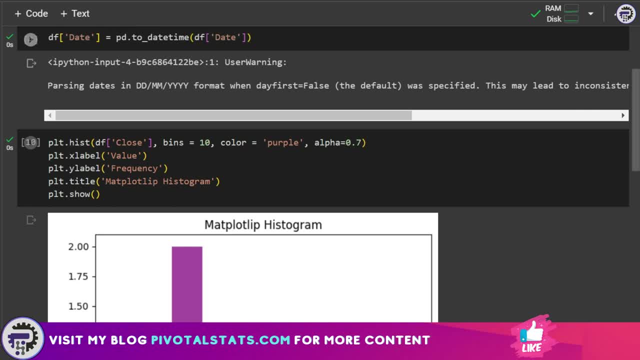 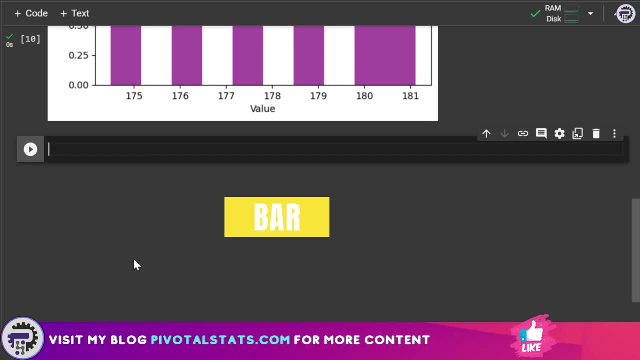 it's advisable to write pltshow, So I'm going to just write that. So this is how you create a histogram using the matplotlib library. Now let's create a barplot using matplotlib. So I'm going to say pltbar, and then I'm going to add a title here, So I'm going to say pltshow. 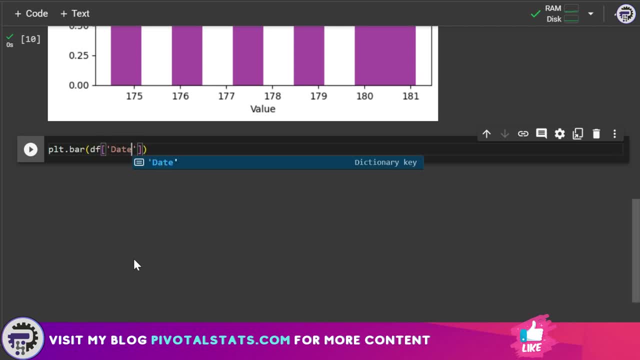 So this is how you create a histogram using the matplotlib library. Now let's create a barplot using the matplotlib library, And then I'm going to use the date column as my x-axis and close column as my y-axis, And then I'm going to assign a color, let's say green. 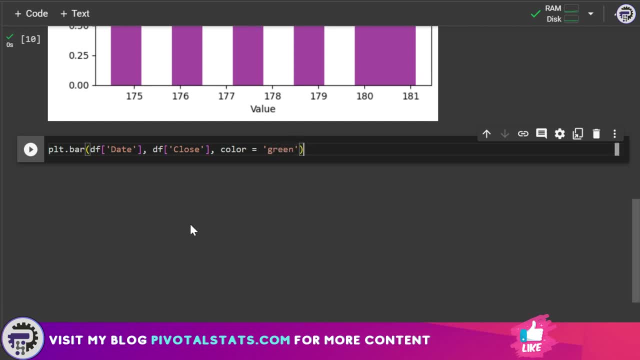 And then, if you choose, you can use the same methods that we used above, which is, you know, add a label to my x-axis, add a label to my y-axis, add a title right. However, for now, I'm just going to continue with just pltshow. 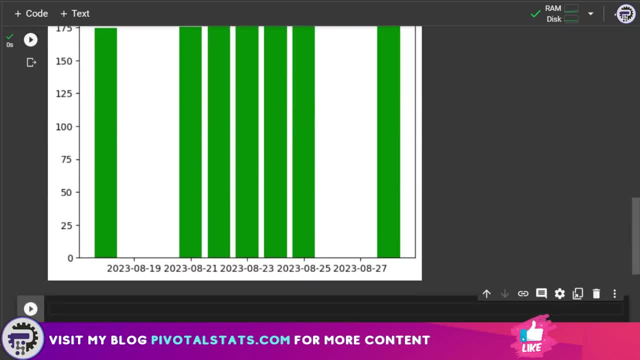 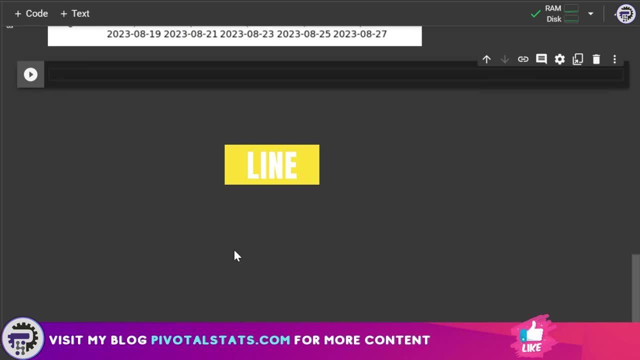 And run this And, as you see, it has displayed my data in a bar chart. now The next one is a line chart. So for line chart you need to write pltplot and then give it a column for x-axis Again, date column for y-axis. 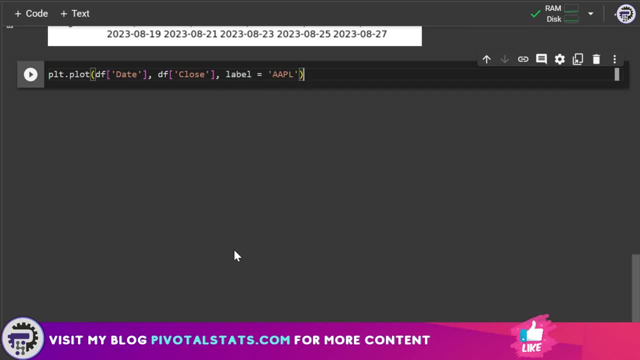 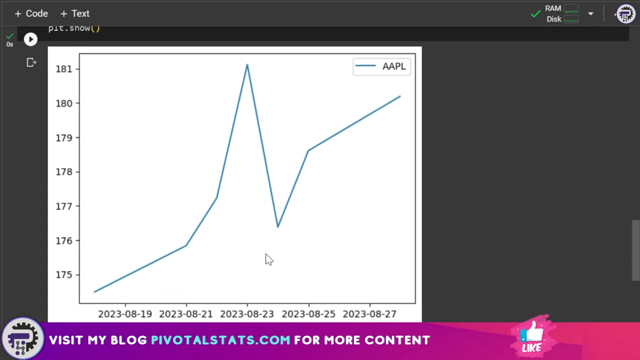 And then this time I'm going to give it a label as well. And again, to customize this chart, you can use x-label, y-label, title. One thing that we have not seen so far is a legend, So let's add that. and then pltshow. So, if you see, it has displayed my data like this. I would like. 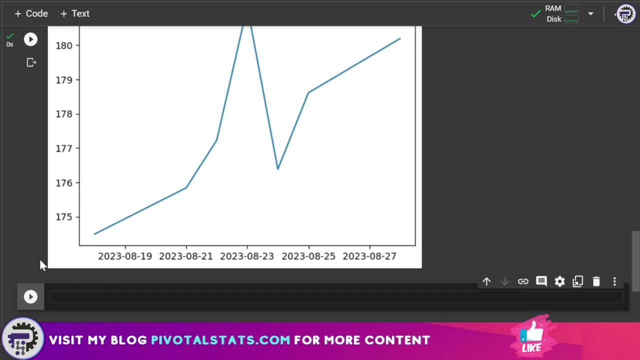 to also mention two important methods that you can use when your x-label is overlapped with each other. So right now, everything is displaying properly, but at times it happens that when you create a chart, the x-label are overlapped. In order to resolve that, you can use two things. 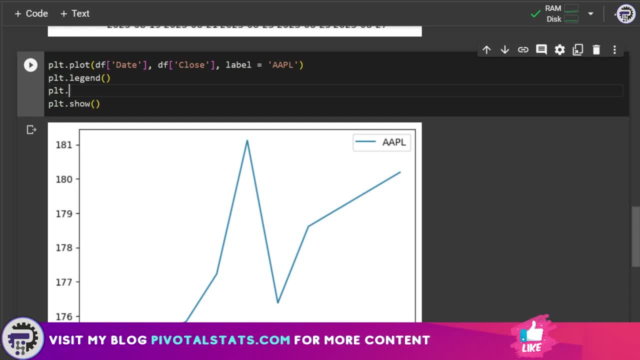 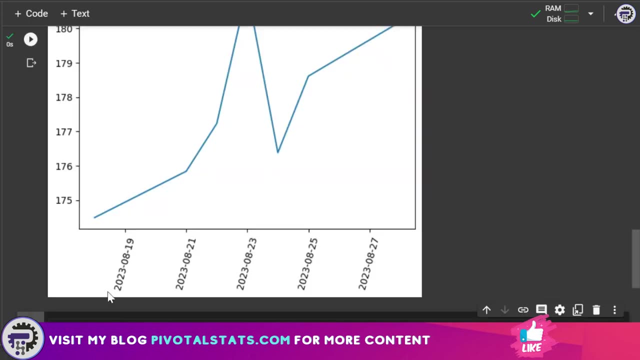 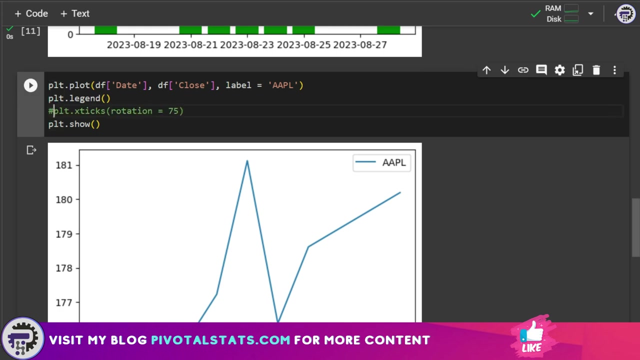 The first one is pltxtxrotation is equal to 75.. What this will do is it will rotate my x-label at an angle. So, as you see, now it is displaying my x-axis like this. Another thing that you can do is if you're dealing with a date column, then you can use this. 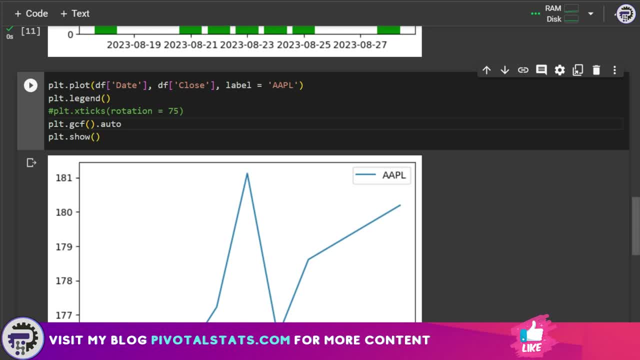 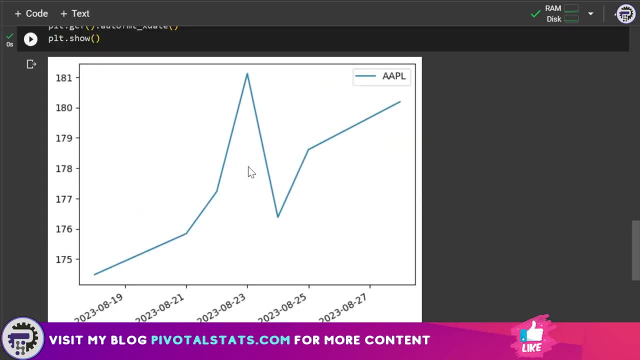 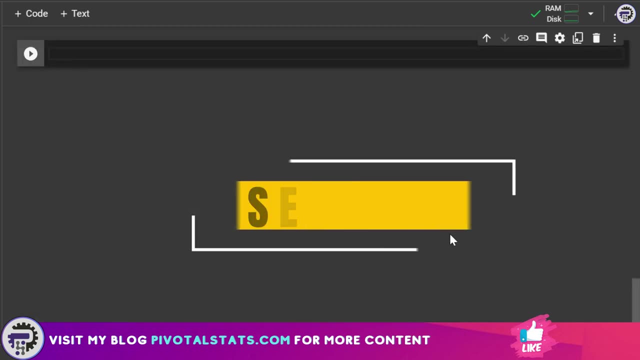 gcfautoformat xdate. Okay, Now, if I run this, this will also automatically adjust my x-labels to format everything properly. Now, the next library we're going to cover is Seaborn. Now, this library is designed to make your visualization more aesthetically pleasing, with minimal effort. 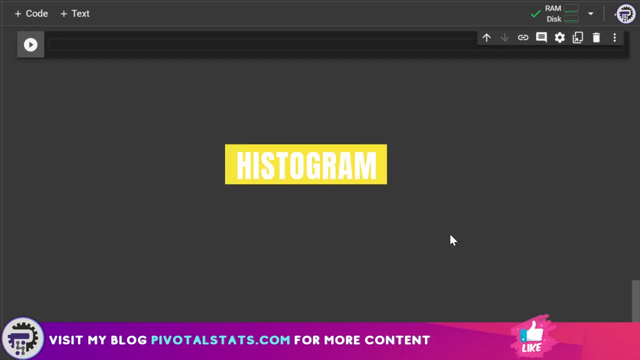 To start with, we're going to create a histogram using Seaborn. If you remember, at the top we have initialized our Seaborn library as sns, So we're going to use that snshistplot. Okay. So this is. 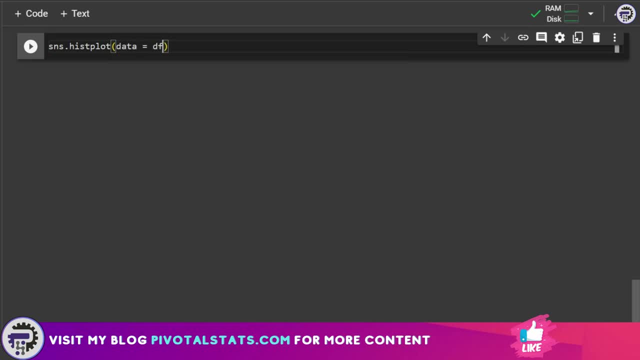 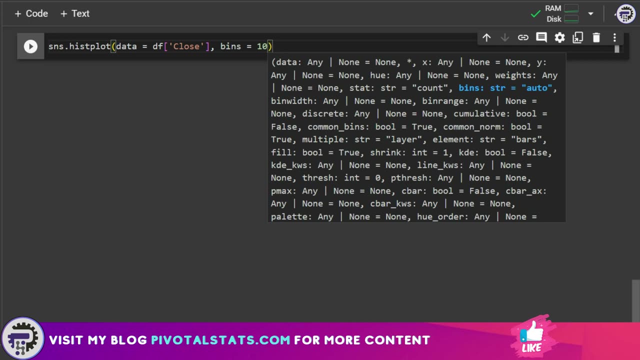 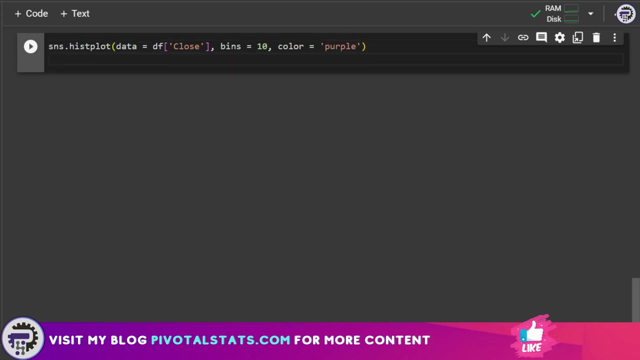 how you create a histogram. data is equal to df- I'm going to use the close column here- bins is equal to 10.. That is the width of my series that I'm going to create And then color. Let's assign a purple color here. Now again, you can use the other methods, like x-label, y-label. 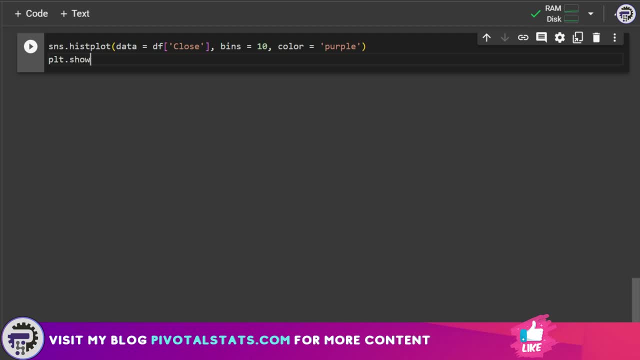 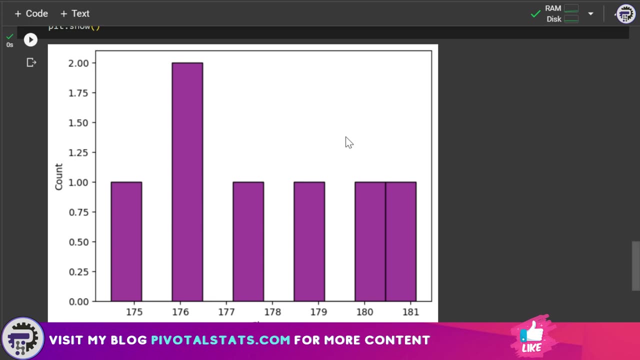 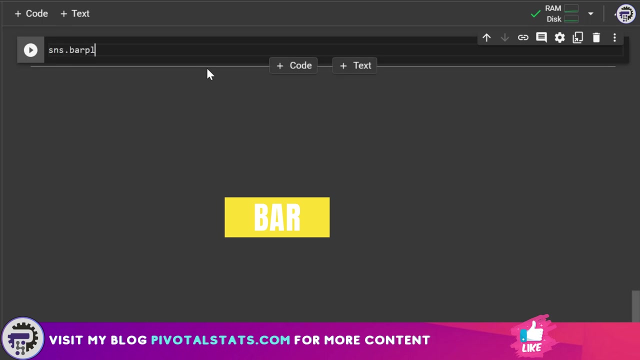 title. I'm going to skip that. However, I'm going to just use pltshow and then run this. Now, as you see, as compared to the histogram created by matplotlib, this is a bit more aesthetically pleasing. Moving on to a barplot, I'm going to use snsbarplot. x is equal to. 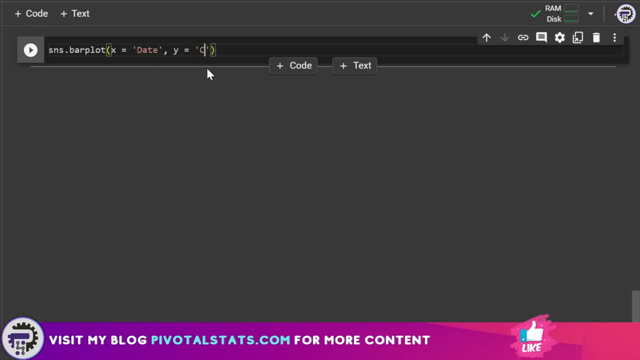 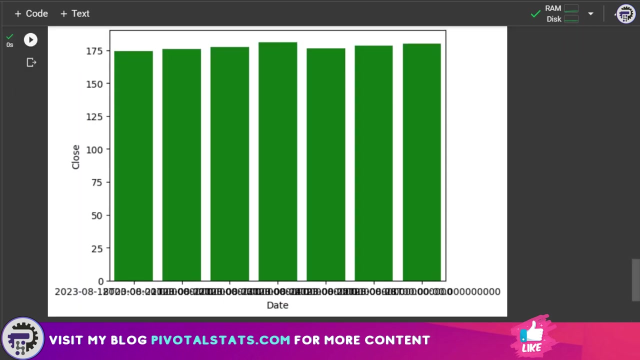 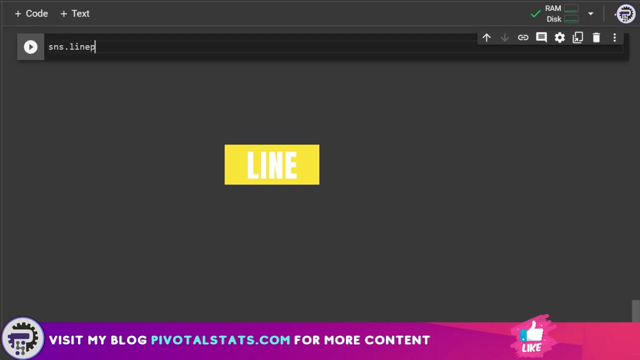 now I'm going to use date. y is equal to. I'm going to use close and data is equal to df Color. let's assign a new color here, green, and then pltshow. Finally, in Seaborn, this is how you create a line chart. So snslineplot x is equal to date column. 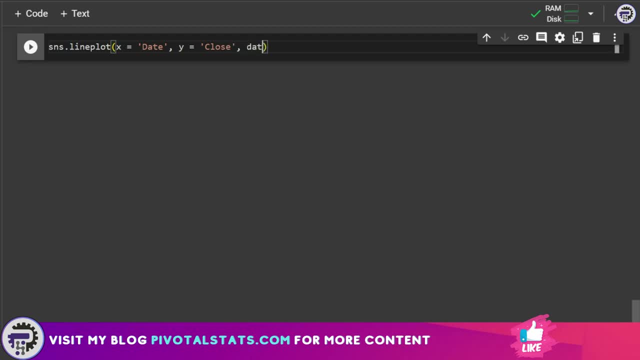 y is equal to close column and data is equal to our data frame, which was df. And then pltshow- Perfect. Now that we have covered the basic charts in matplotlib and Seaborn, let's take a leap into the interactive world of Plotly Now. this library specializes in creating interactive visualization. 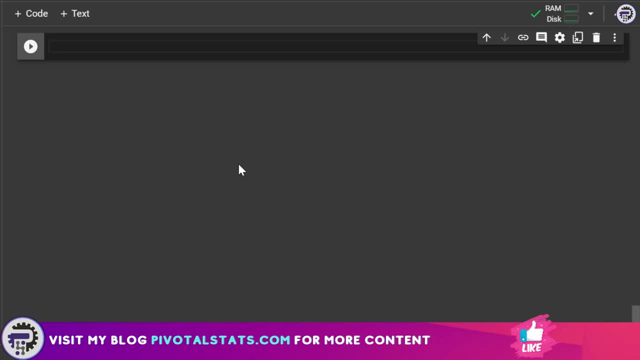 that allow users to explore and interact with data in real time. Now this is perfect for creating web-based dashboards and reports. To start with, let's create a bar chart, So we're going to start with a name. You can assign any name to it. Now, if you remember, we have initialized the Plotly library. 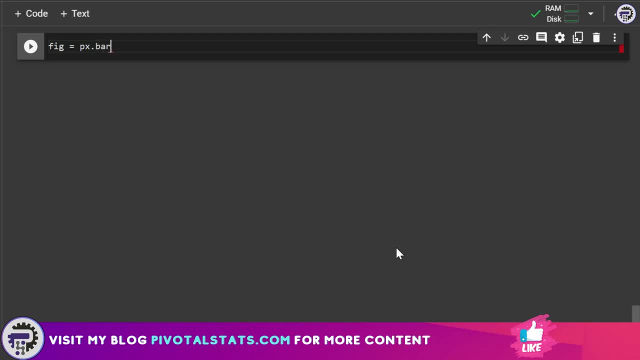 with the initials px. so we're going to use that pxbar because we're creating a bar chart, and df. this is the data frame that we're using: x equal to date, y is equal to close. We can add a title here, and then, finally, I'm going to say figshow. 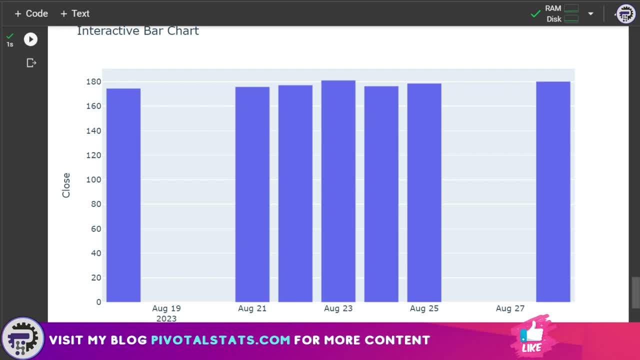 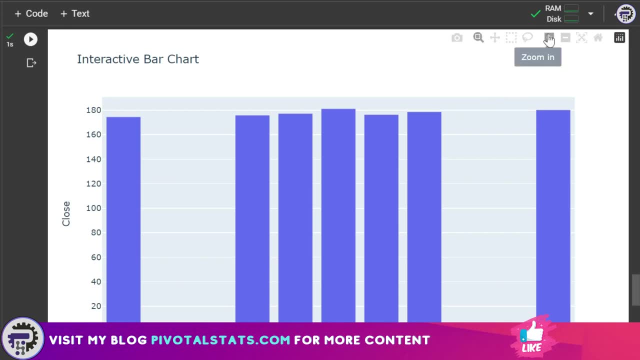 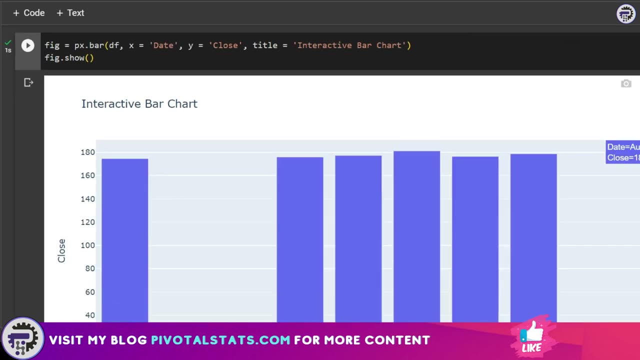 With just two lines of code, it has created an interactive chart with much better visualization. now the important part here is this chart is interactive, so there are a few options. if you see here, you can zoom into the chart. we can also highlight a certain portion of the chart like this and then zoom into that so that you can. 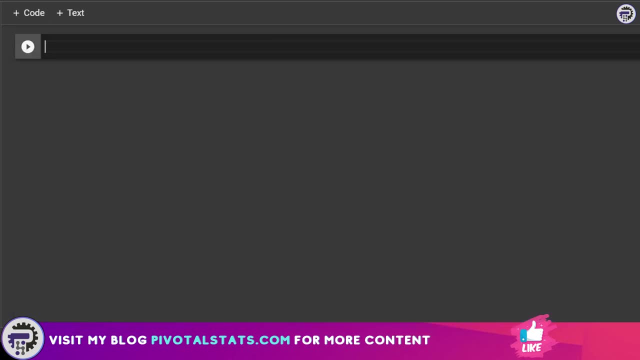 play around with the data and dig deep into the charts. now let's create a 3d scatter plot. so I'm gonna use: fig is equal to P, X, dot scatter underscore 3d, and then DF, X equal to date, which is my x-axis. y is equal to close, and then I'm 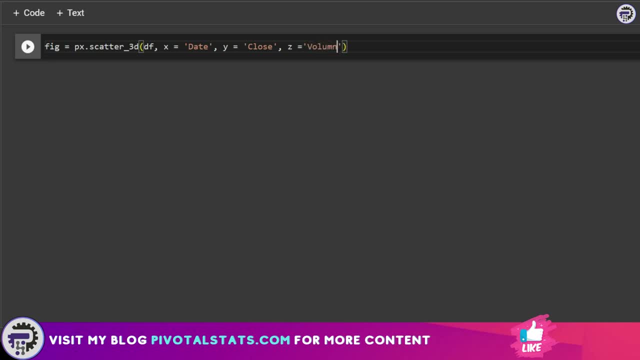 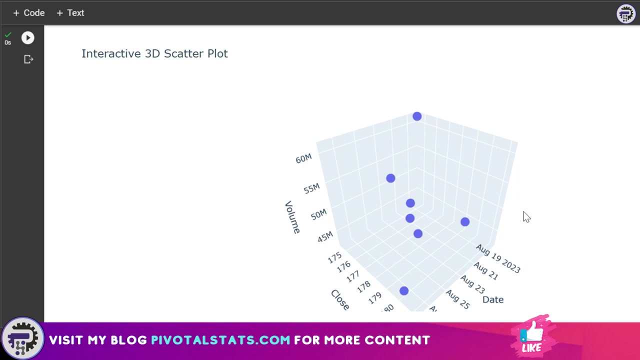 gonna assign a z-axis as well. this case I'm gonna use volume column and then let's assign a title. finally, fig dot show. now, if you see, if this chart is completely interactive, user can input with this chart and see this chart from various angles, although there may be better use cases for this chart in different type of data. now, 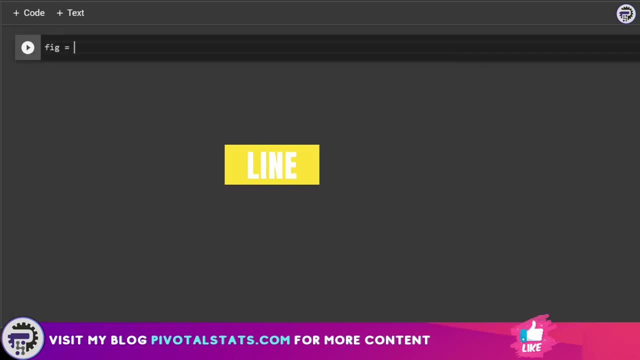 let's create a line chart with plotly. so fig is equal to P, X dot line, and then DF, X equal to date, Y is equal to. I'm gonna use two columns here, just so that we can compare both columns together. I'm gonna use Global andwarmirata function, so double eachЬ. all that will go away. so this is my. 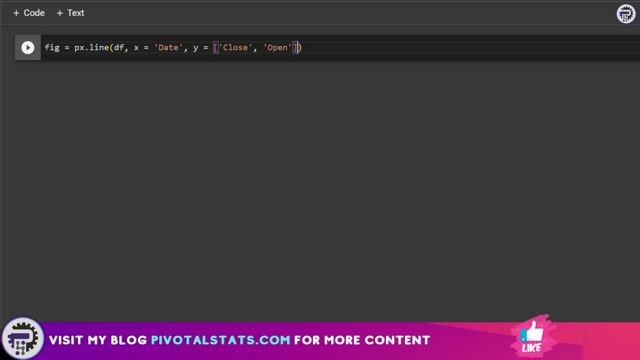 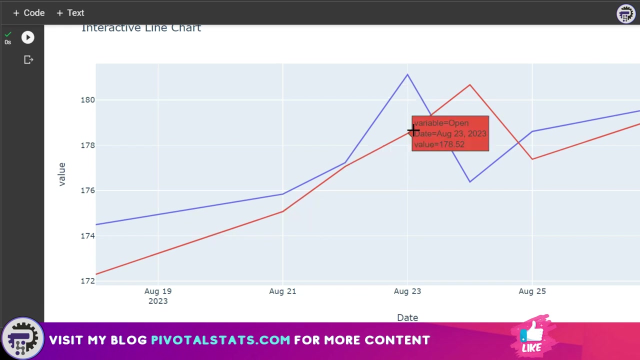 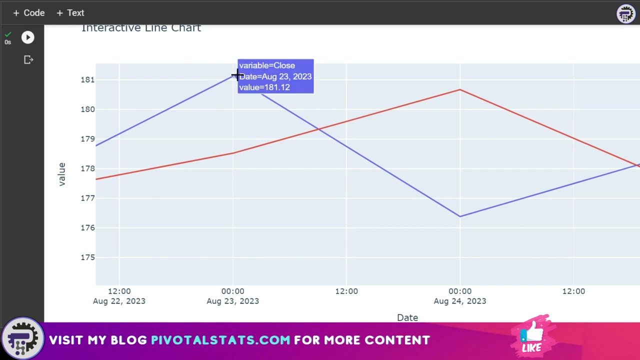 closing column here and the open column here, assign a title and then right click dot show. now, if you see, we've created a line chart comparing the opening price and the closing price of share on each dates and if i want, i can zoom into a certain part of the chart and see further details. 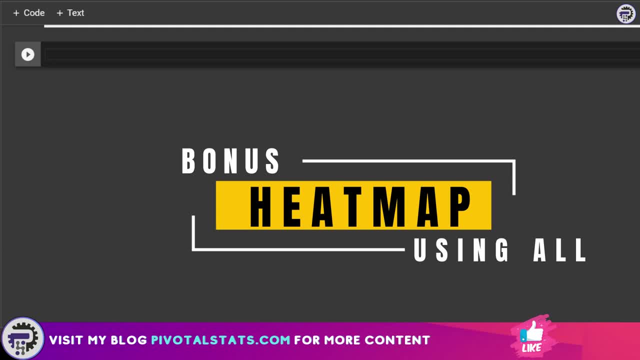 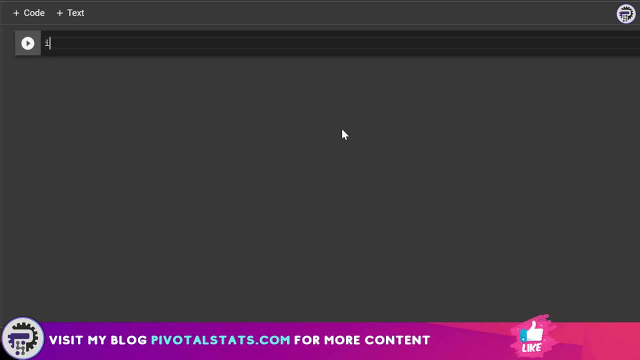 now, finally, for those who have stayed till the end, this is how you create a heat map using all three libraries. so for this, i'm gonna create a data using numpy library. so i'm gonna import numpy, okay, and i'm gonna create a random data. once that is done, i'm going to create the charts using all three libraries. 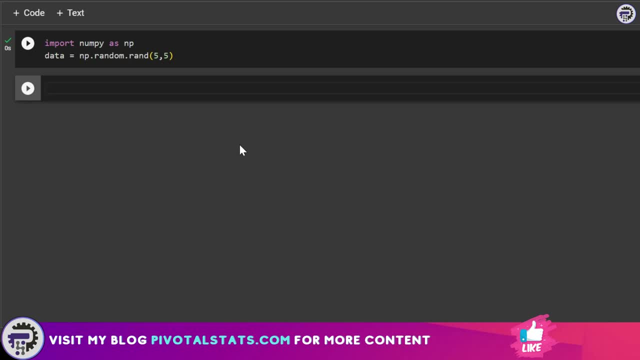 now, this is how you can create a heat map using matplotlib. so plt dot imshow data cmap equal to viridis. okay, now it is just color palette that we have, so we're going to use that color palette and we can have additional methods here. so plt dot color bar. 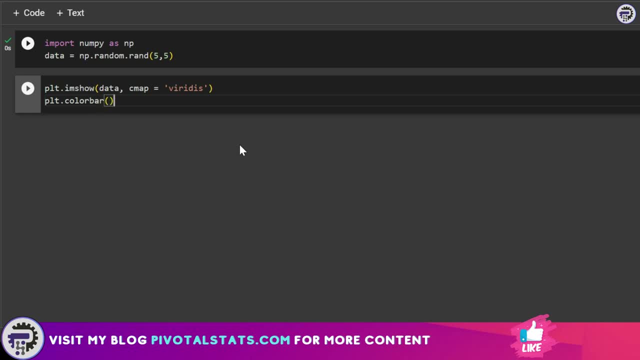 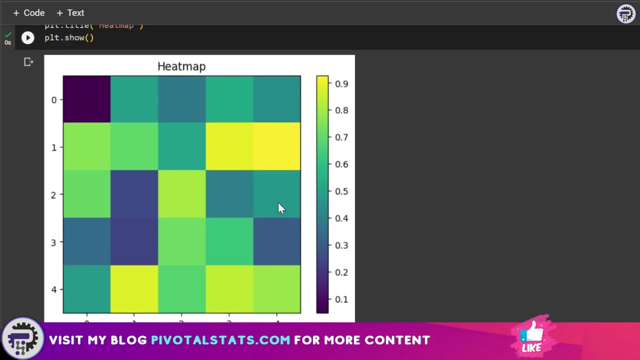 will add a color bar to the right of the chart. we can have the title and then write plt, dot, show. if you see, this is how you create a heat map using matplotlib. okay, now the same thing can be achieved using a seaborn library. so i'm going to say: 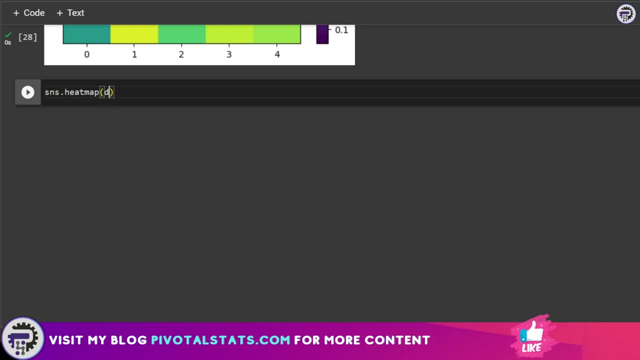 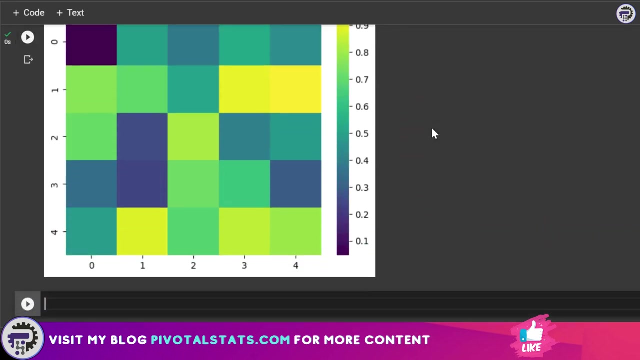 sns, dot heat map data, cmap is equal to, again, viridis. i'm going to skip the title part or other methods for now and i'm going to say plt, dot, show. so if you see, the line of code that i've written here is much smaller. however, the output is more or less. 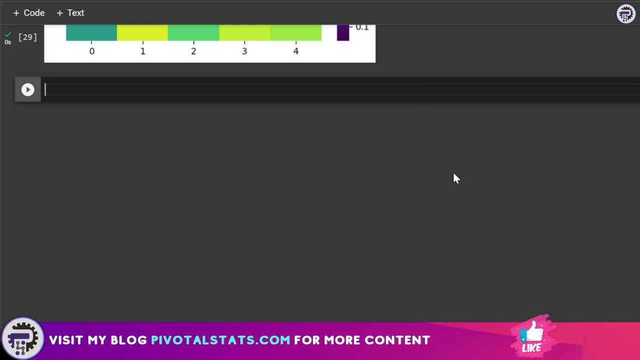 the same. okay, finally, a heat map using plotly. i'm going to say: fig is equal to px. dot imshow data color underscore: continuous scale is equal to viridis. this is equivalent to the color bar map parameter that we have given earlier. and then i'm going to say: fig, dot show. 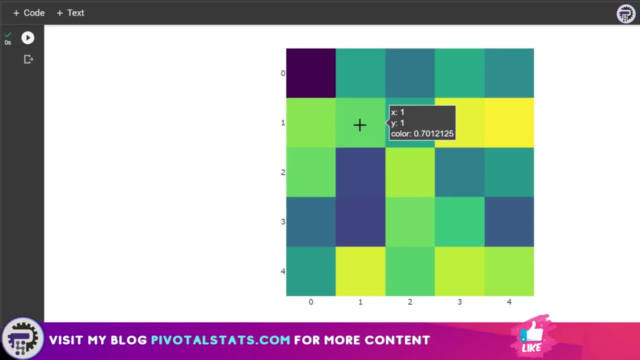 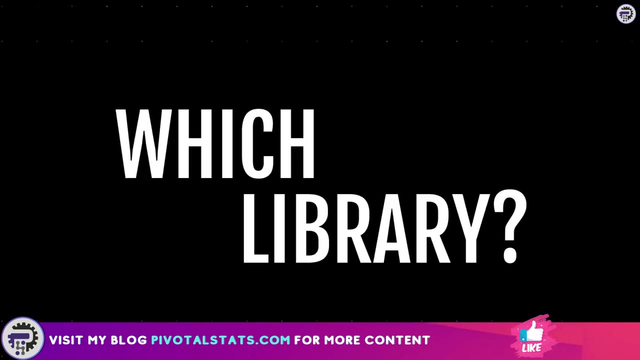 okay, so it created a chart. however, because we are using plotly, this is interactive. i can select this and zoom into that particular portion of the chart. so, now that you have seen all the visualization, which library to choose is completely up to you. matplotlib is for foundational static plots.